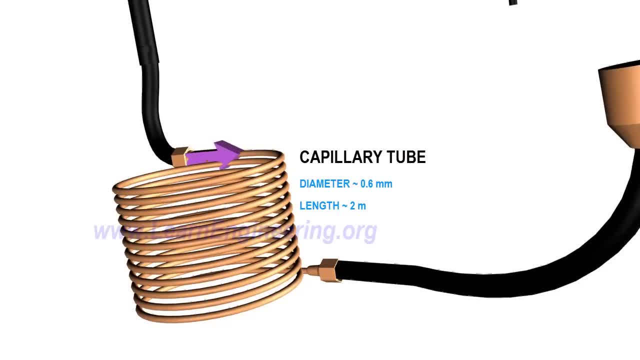 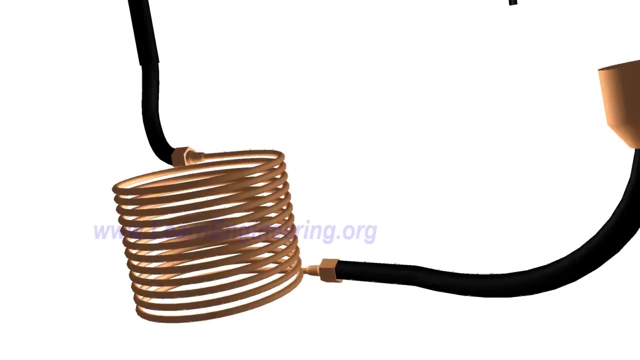 Throttling device is an obstruction to the flow which causes tremendous pressure drop. Due to drop in pressure, boiling point of refrigerant comes down and it starts evaporating. Heat required for evaporation comes within the refrigerant, so its temperature drops. 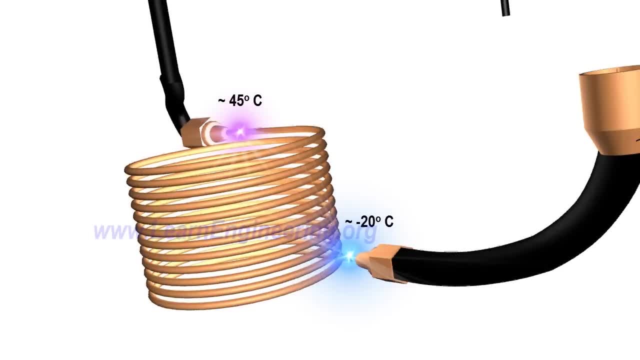 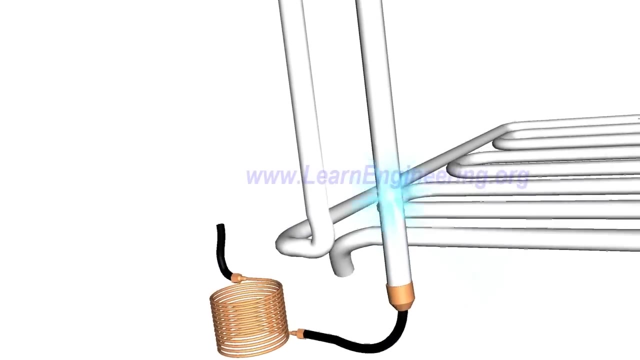 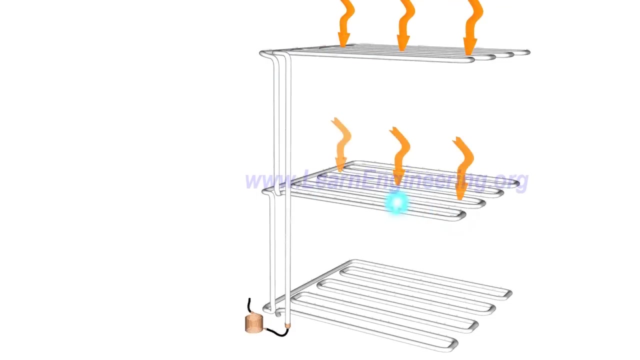 If you check temperature across throttling device, you can notice this drop. Next phase is simple: Just pass this cold liquid over the body where you have to absorb heat. During heat absorption process, refrigerant further evaporates and transforms into pure vapor. 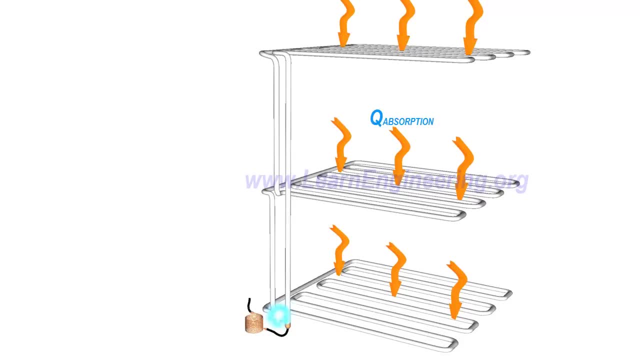 So we have produced the required refrigeration effect. If we can take this low pressure vapor refrigerant to state before throttling process, that is, high pressure liquid state, we will be able to repeat this process. So first step, let's raise the pressure. 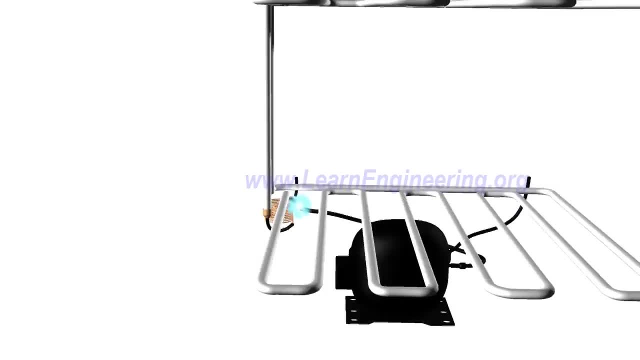 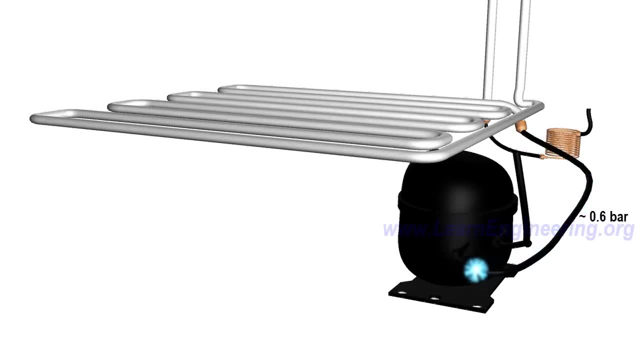 A compressor is introduced for this purpose. Compressor will raise the pressure back to its initial value, But since it is compressing, gas, along with pressure, temperature will also raise. It is unavoidable- Now the refrigerant is high pressure vapor To convert it to liquid state. we are introducing another heat exchanger. 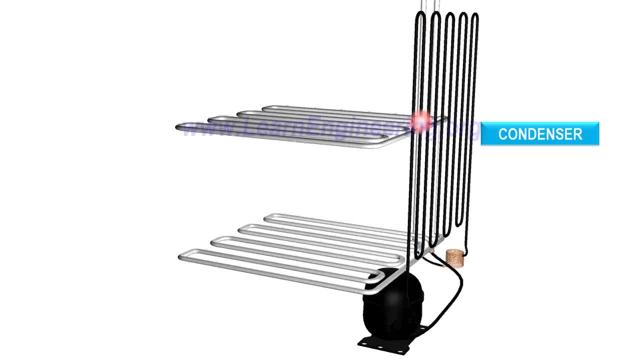 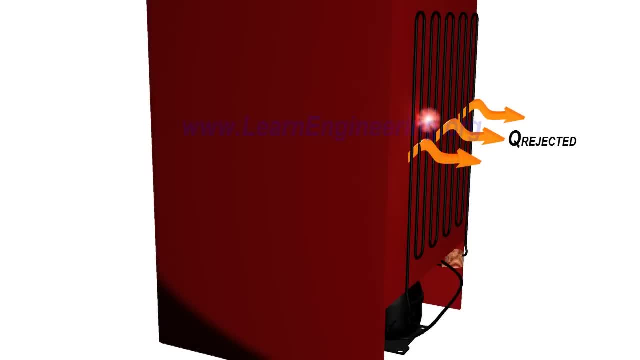 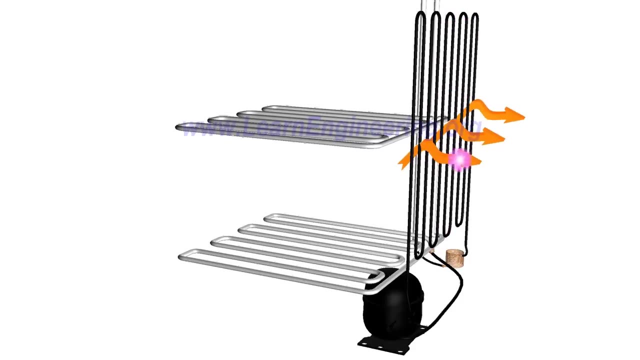 This heat exchanger is fitted outside refrigerator So it will liberate heat to the surroundings. Vapor will get condensed to liquid and temperature will come down to normal level. So the refrigerant is back to its initial state again: high pressure liquid. 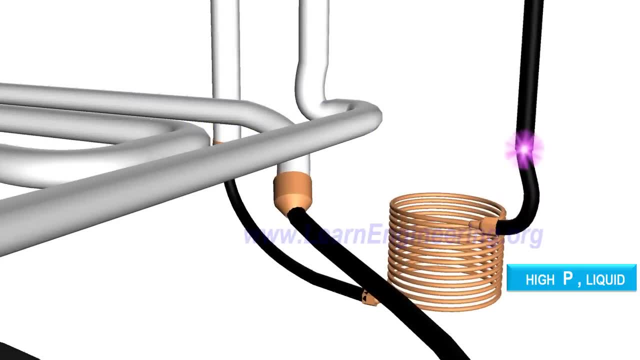 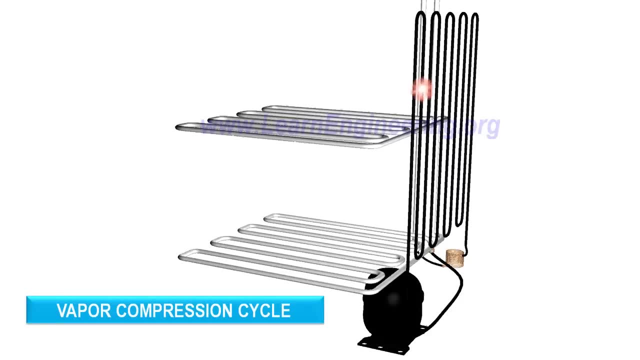 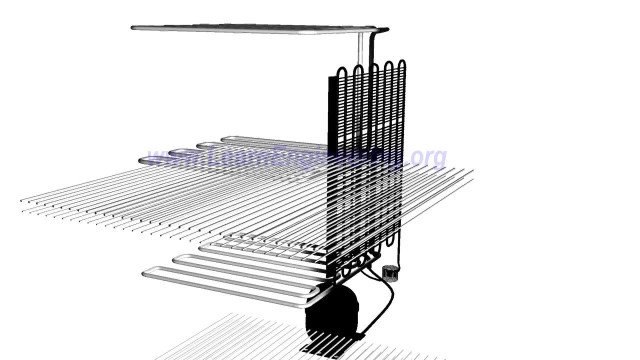 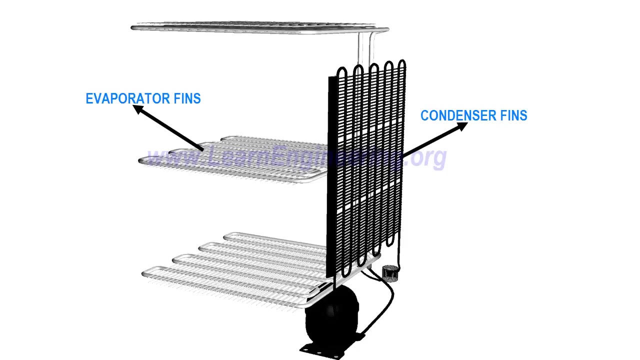 We can repeat this cycle over and over for continuous refrigeration. This cycle is known as vapor compression cycle. You can note more details of refrigerator components here. To enhance heat transfer, both evaporator and condenser are having fins attached to it. Since evaporator is cooling the surrounding air, it is common that water will get condensed over it, forming frost.